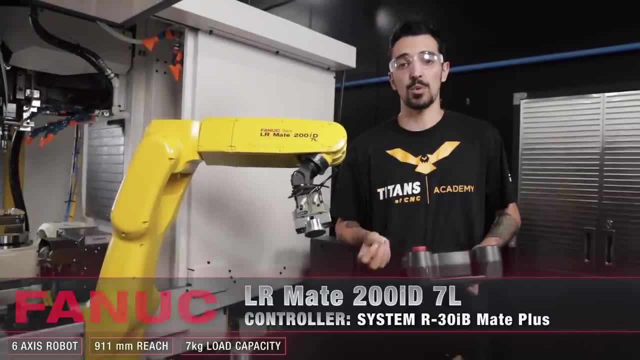 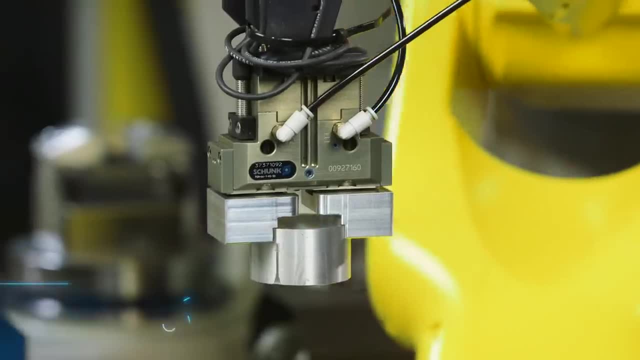 What we're going to be doing is just going from a point A position, where I'm going to have a puck, and go into a point B position, which is my pneumatic vice inside of my machine, and placing it inside. When it comes to our end effector on our robot, we have a PGN plus 64 and our machine. 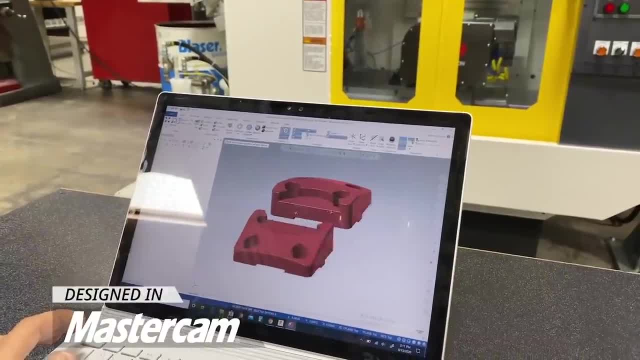 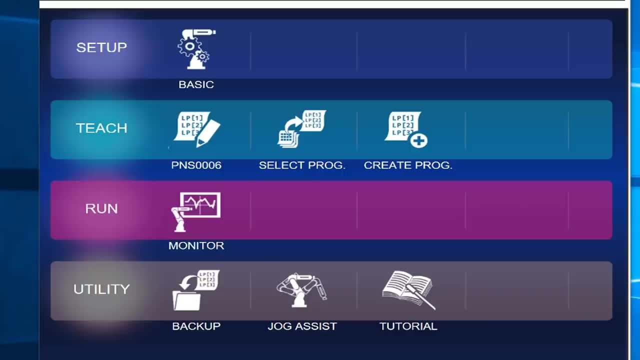 jaws that you may have seen in a previous video, where we started with 3D prototypes and this is what we got for our production. So now that you know all that, let's get after it. This is going to be the home screen for your Fennec Teach Pendant, which comes with the LR Mate robot and 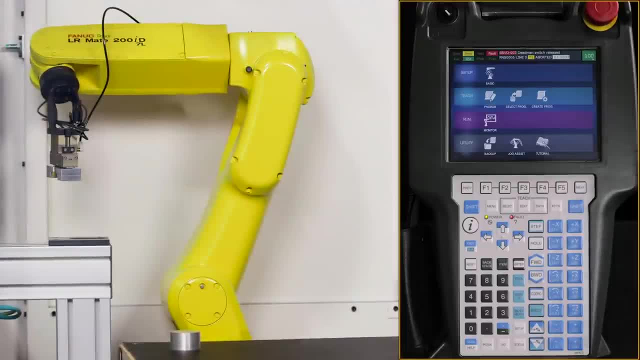 all other models of robots that Fennec has. From this page we're going to hit the select button, and that select button brings us directly to where we hold all of our programs that are on our Teach Pendant, and from here we're going to need to create a brand new program so we can. 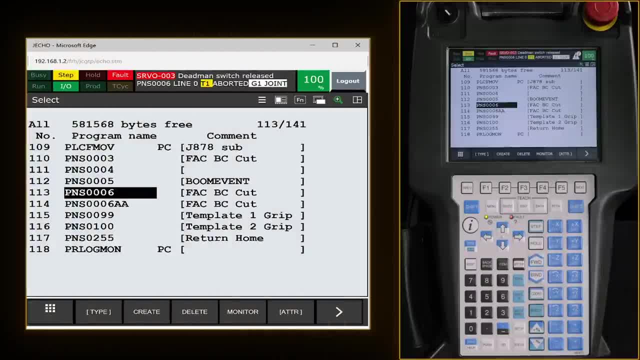 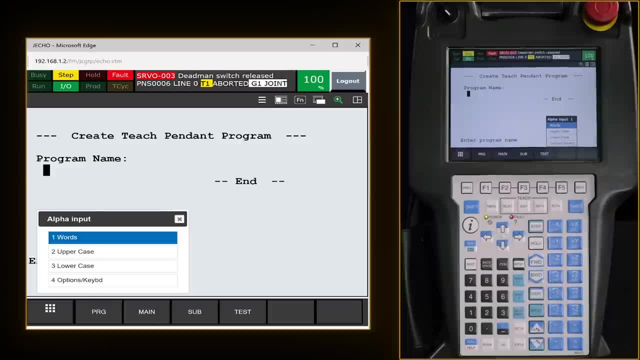 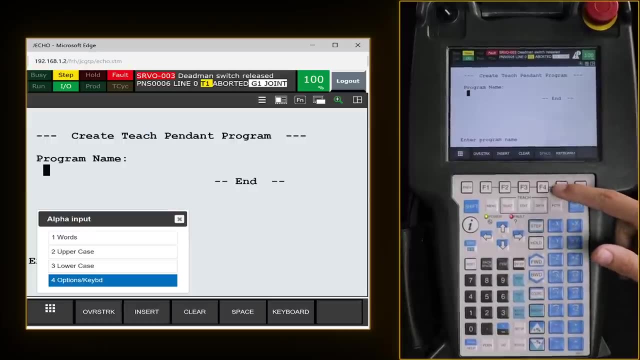 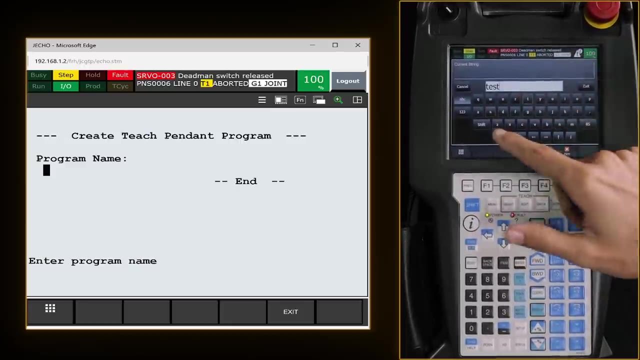 start plotting points. F2 is going to be our create button. Now, from here we need to give our program a name. I like going down to the options and keypad so I can hit F5, which is keyboard, and from here we can give it a name. For video purposes, we can put test one one, since 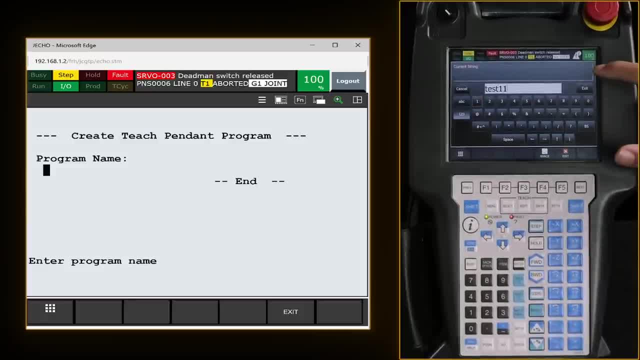 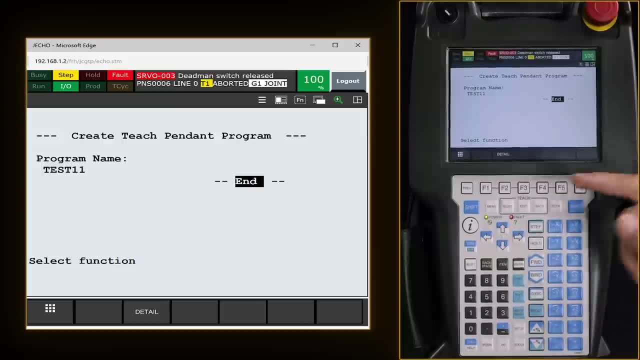 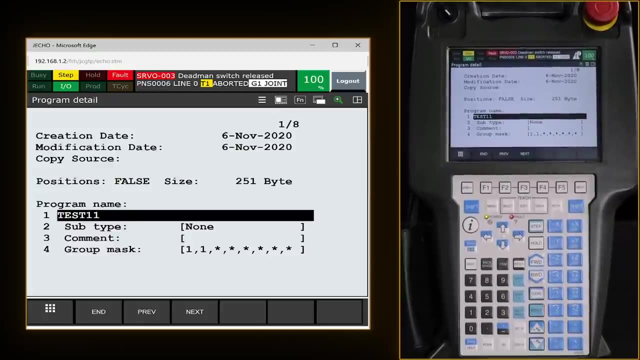 we're doing it in November. Once you figure out your name, we're going to hit exit. You can see it populate right under program name and from here we're going to hit F2, which is detail. Now, the only thing that we really have to worry on this screen for right now is going down to group. 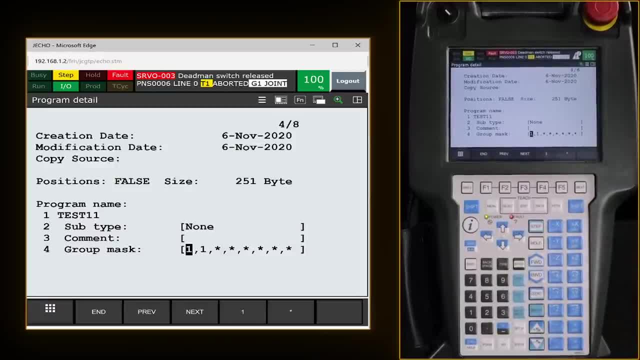 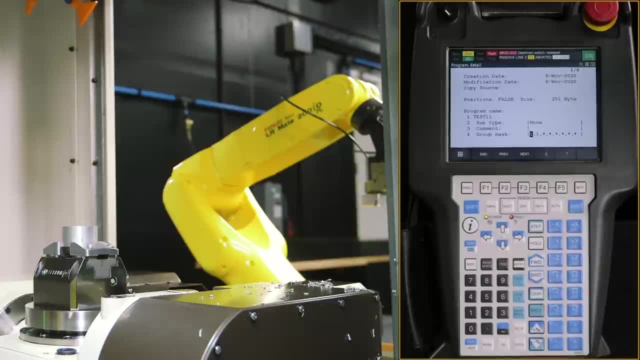 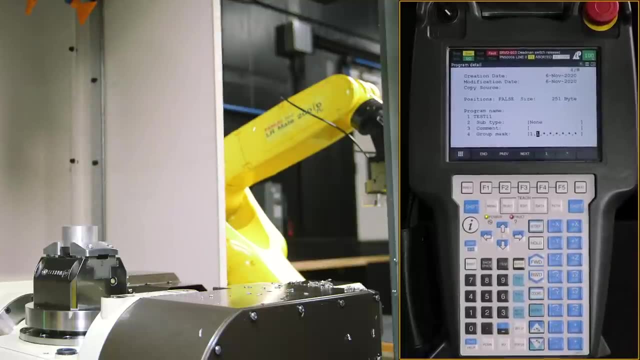 mask, and what these two ones are is basically when you have multiple groups, So our robot in itself is group one. We have a servo door on our robo drill, which would be the second one, And since we're not going to be utilizing both of those at the same time in this video, 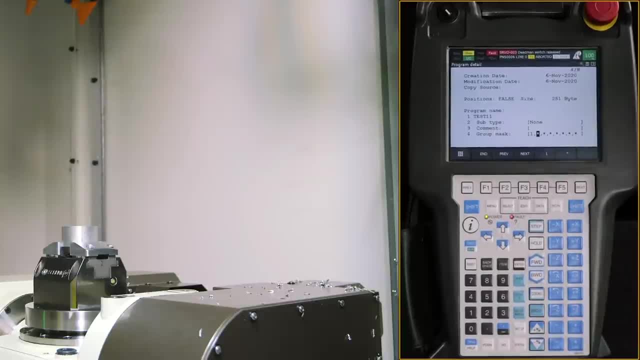 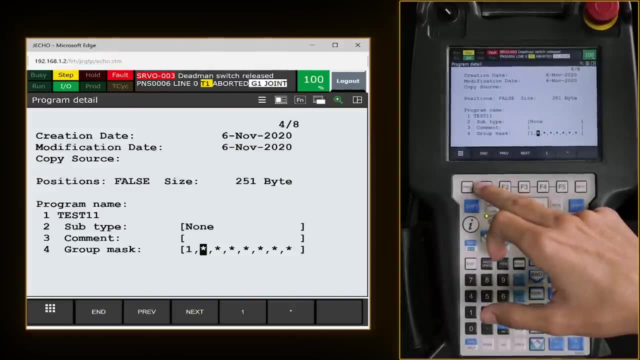 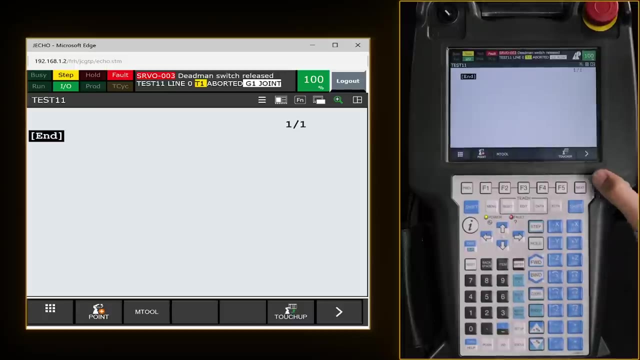 we are going to set that to an asterisk, which is F5, and so now we'll just be working around the arm itself. Once we're done with that, we can hit F1, which is end, and now we're ready to start adding points From here. what I like to do is hit our next key, which will arrow over, and hit F5 for edit. 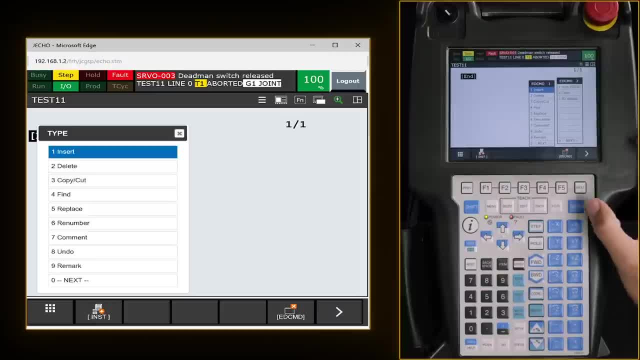 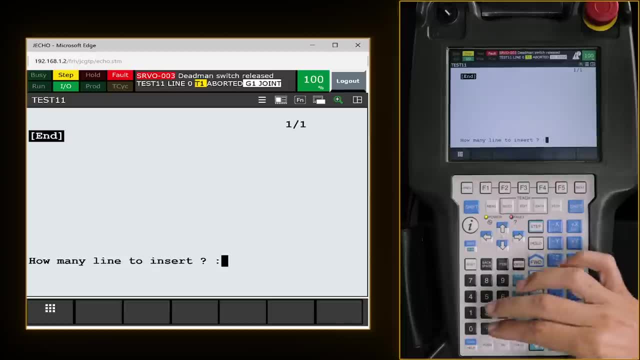 and I just like inserting by hitting enter. I'm going to hit enter and it's going to ask us how many lines we would like to enter. I just give myself some space, so I will put in 10, enter. Now. the first thing that we can do is open. 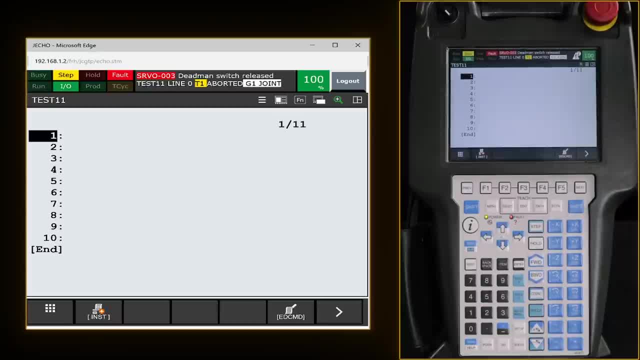 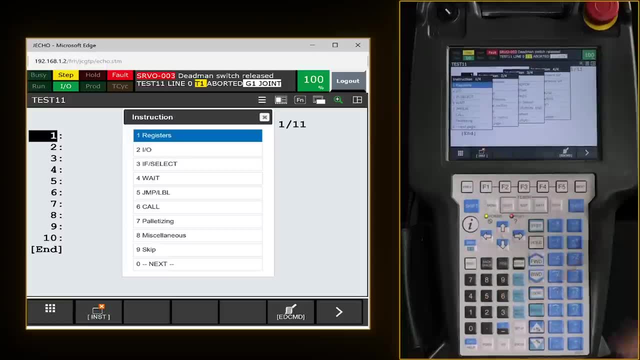 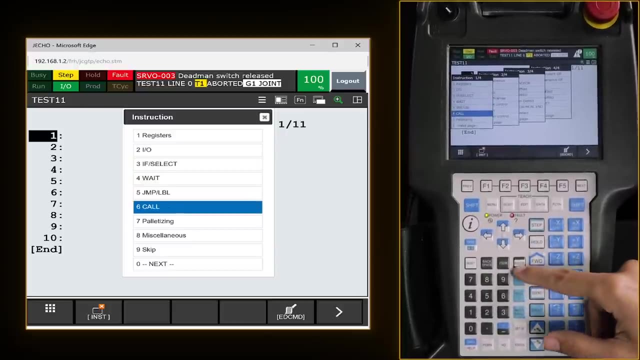 up our servo door so we have a lot more mobility when it comes to moving our robot arm. To do this, we're going to go to F1, which is insert, and we are going to actually call the open door program by going down to six. 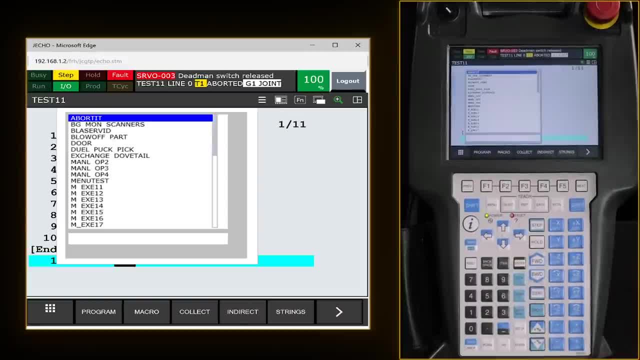 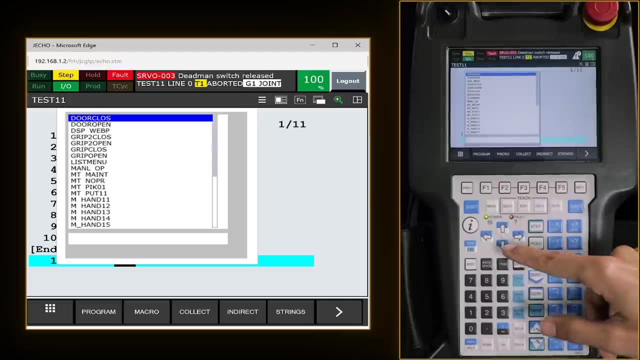 Hitting enter, we're going to select call program and now it's asking us: what do we want to do? So we're actually going to go over to F2, which is a macro settings. So these are all of our macros that you can customize. We have a door open and door closed for the servo. We are going to go to. 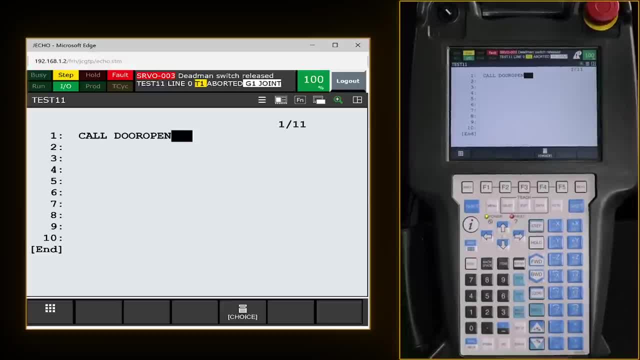 door open, enter and boom. right there we have our first line of code for our robot program and it is called door open. Once we put it in, we actually want to utilize it to open our door so we can start moving our robot around to get our point pickups. To do that you need to press on your dead man in the back. 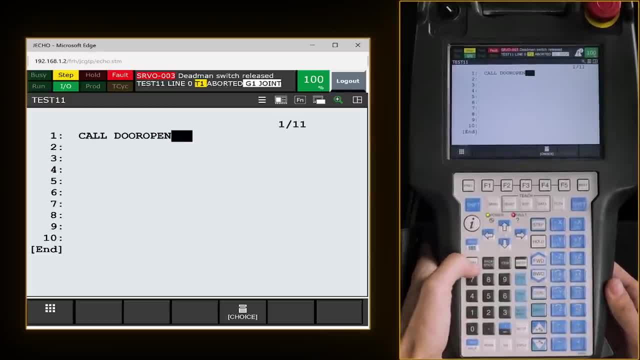 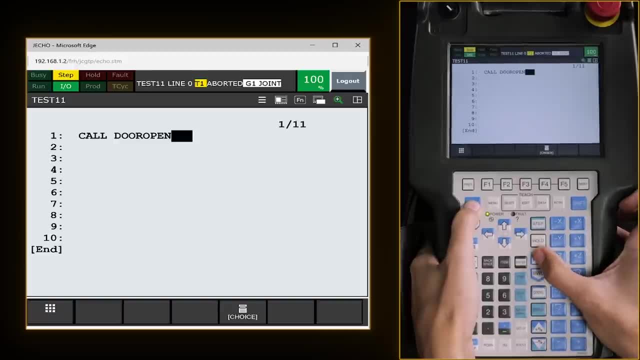 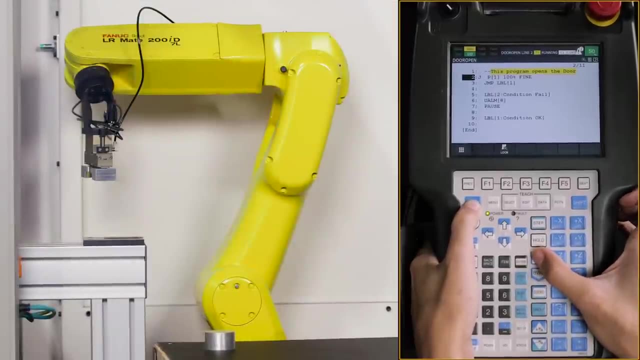 If you have a dead man switch release alarm you need to hit reset. There's no faults. so now we can hold shift forward and it goes to the macro program to open our door. So we're going to hit forward until our door opens and it's going to stay on line two until 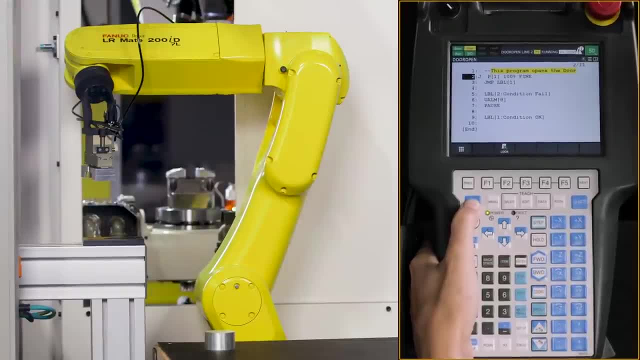 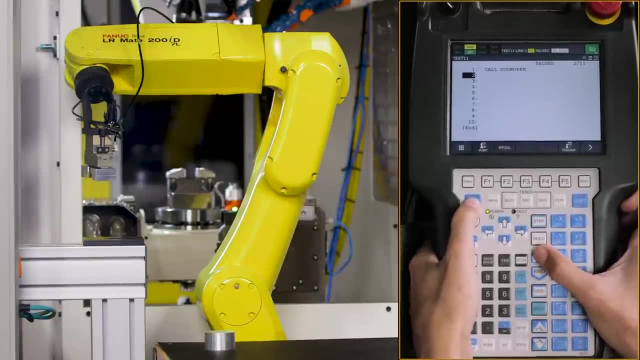 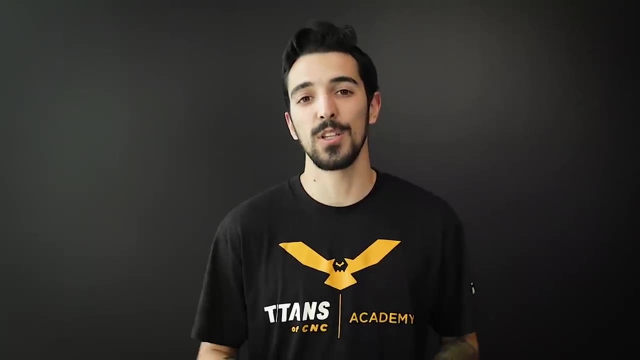 the door fully opens to what we programmed it to previously. Now that it's open, we will keep hitting forward until it gets out of the macro program and we are now back in our code to write our program. All right. so after following those steps, what you'll have now is a robot program that is ready. 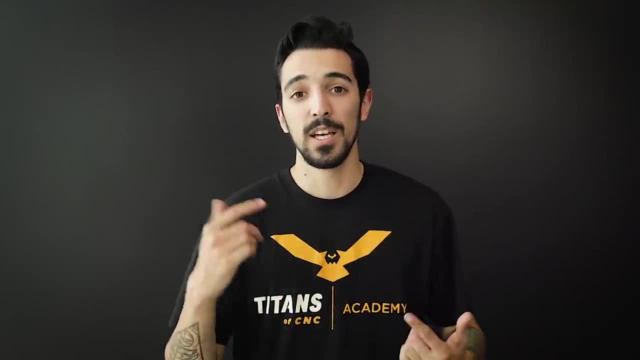 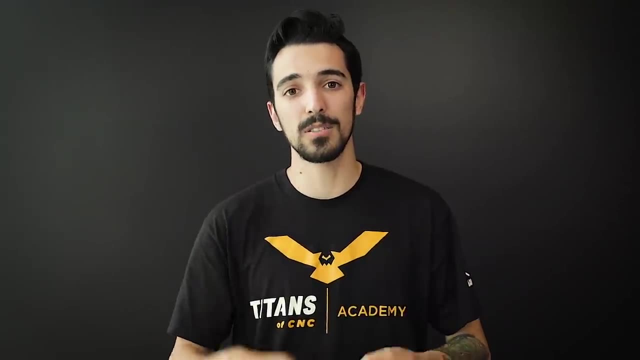 for you to add in your codes to get things done- Things moving. in our next series of videos we're going to have things showing you how to move the robot arm. We're going to show you how to pick and place parts. We have pneumatic vise, so your machine.